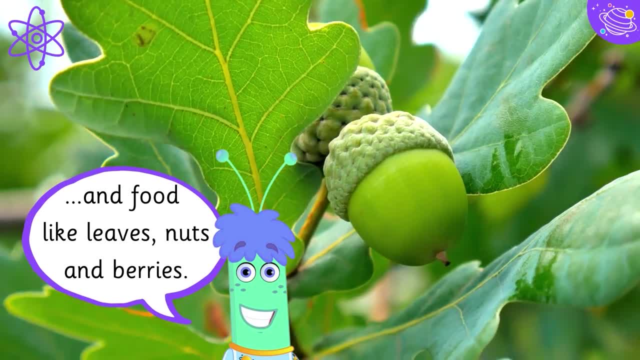 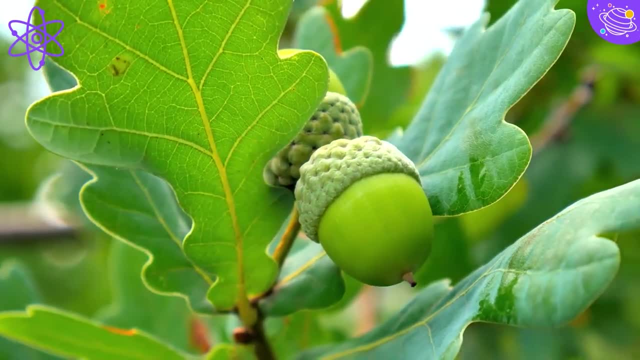 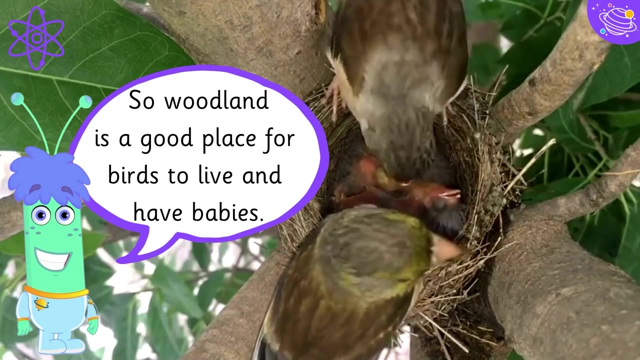 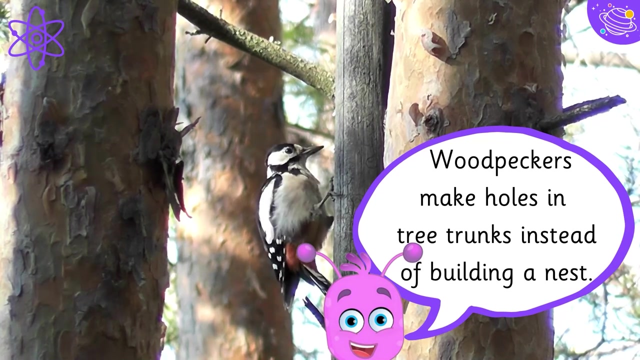 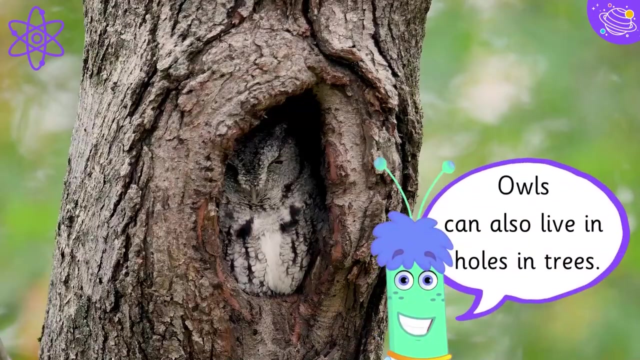 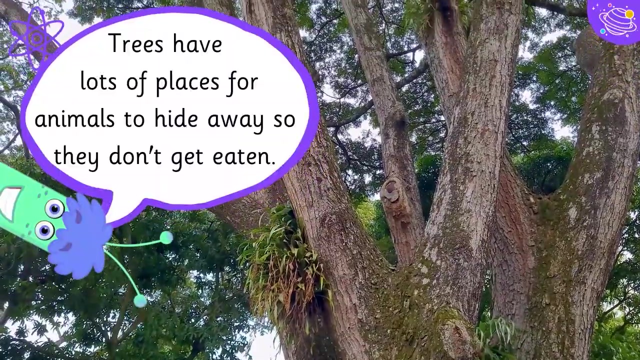 And food, like leaves, nuts and berries, So woodland is a good place for birds to live and have babies. Woodpeckers make holes in tree trunks instead of building a nest. Owls can also live in holes in trees. Trees have lots of places for animals to hide away, so they don't get eaten. 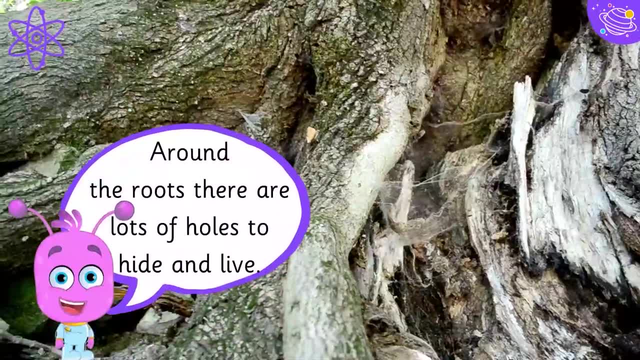 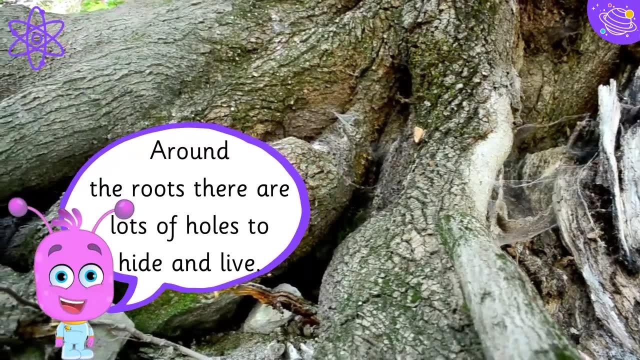 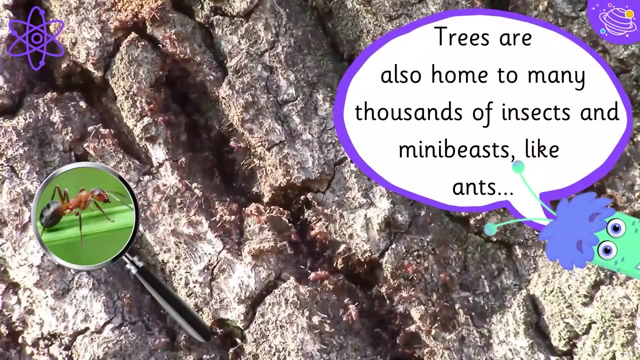 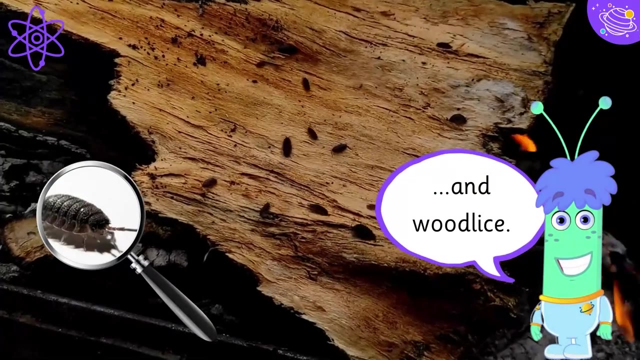 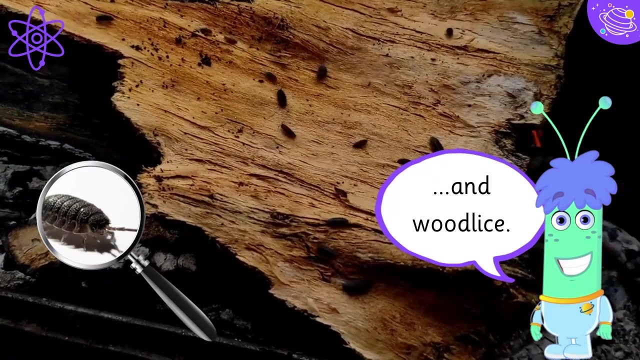 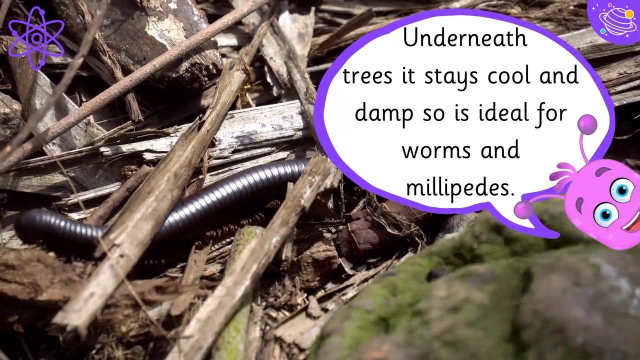 Around the roots there are lots of holes to hide and live. Trees are also home to many thousands of insects and mini beasts like ants And wood lice. Underneath trees it stays cool and damp, so it's ideal for worms and millipedes. 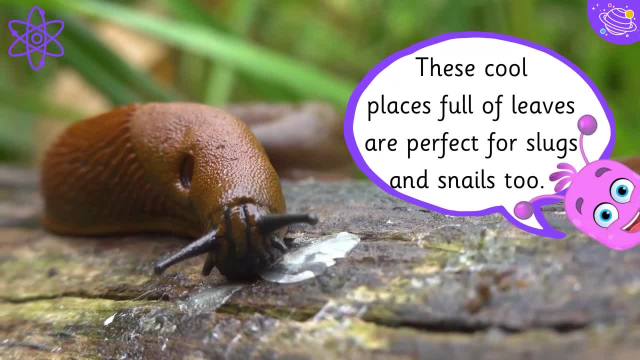 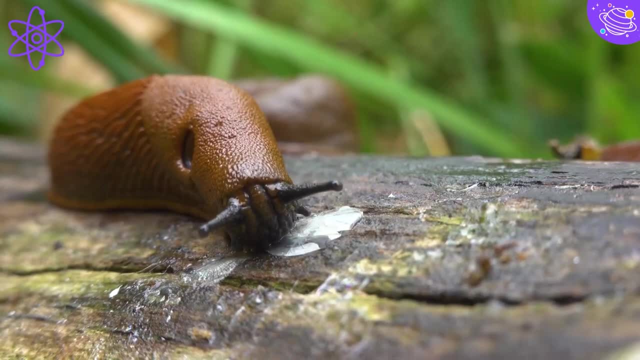 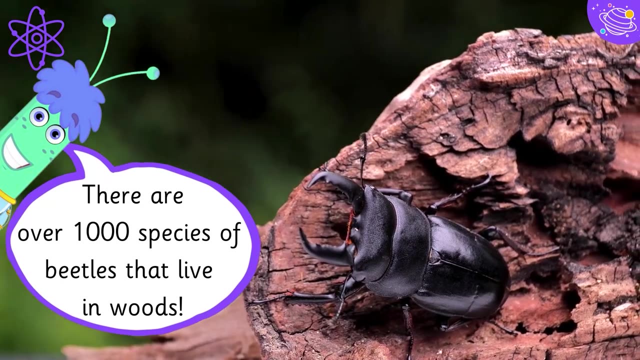 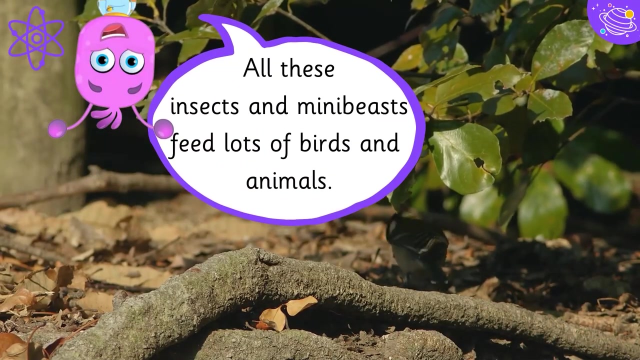 These cool places full of leaves are perfect for slugs and snails too. There are over 1,000 species of beetles that live in woods. All these insects and mini beasts feed lots of birds and animals. All these insects and mini beasts feed lots of birds and animals. 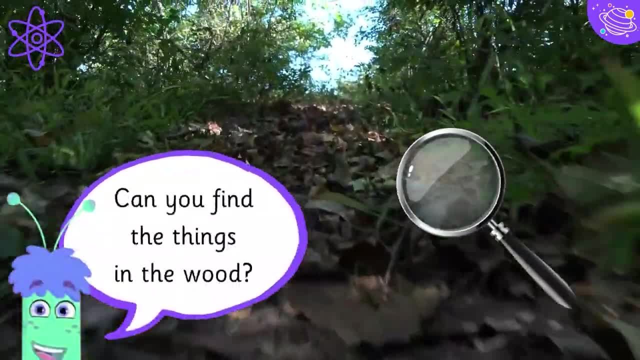 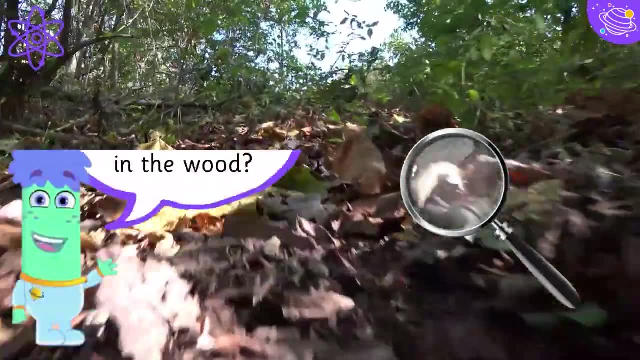 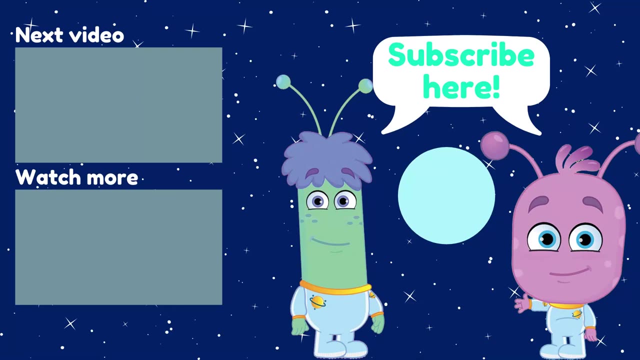 Not only in restaurant, encouraging resonance of woodiskt, they also feed some other creatures. Wood può salutare. Can you find the things in the wood Well done? Goodbye, Good bye you.